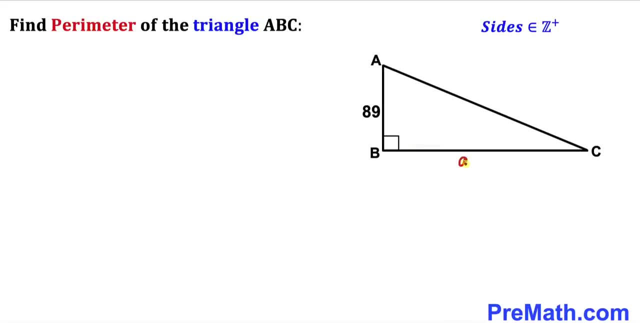 first I'm going to call this side length lowercase a, this side length lowercase b and this longest leg as our side c. And now we are going to use the Pythagorean theorem. And here's our Pythagorean theorem: a square plus b square equal to c square, where our this horizontal side length 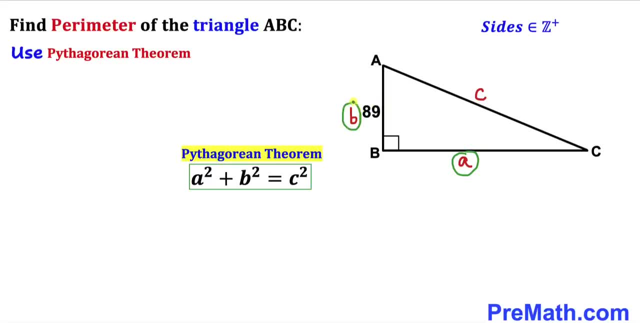 is lowercase a, our vertical length is lowercase b and our hypotenuse is c. So let's go ahead and fill in the blanks. in this Pythagorean formula, Only thing that is known is b equals to 89. So therefore, let's go ahead and fill the blanks. a square plus 89 square equal to c square, Let's. 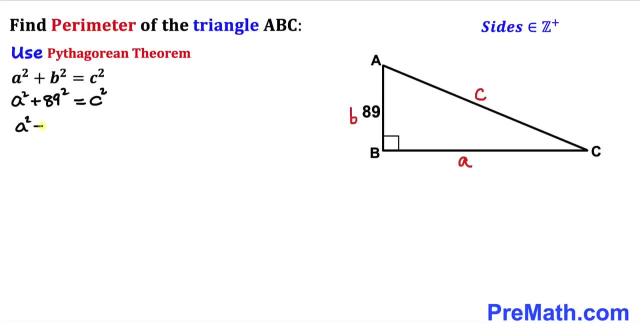 go ahead and simplify, So that is going to give us a square plus b square, equal to c square. So plus 7921, equal to c square. let's move this a square on the right hand side, so therefore we're going to have 7921 equal to c square minus a square. and now this equation could be written: 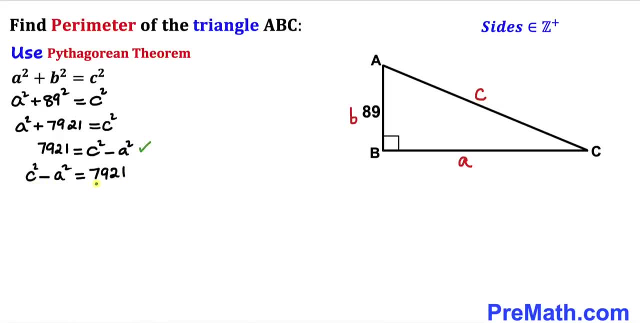 as the other way around: c square minus a square equal to 7921, it doesn't make any difference whatsoever. and now let's recall this famous identity: a square minus b square, that is, means the difference of two squares could be written as the product of sum and the difference a plus b. 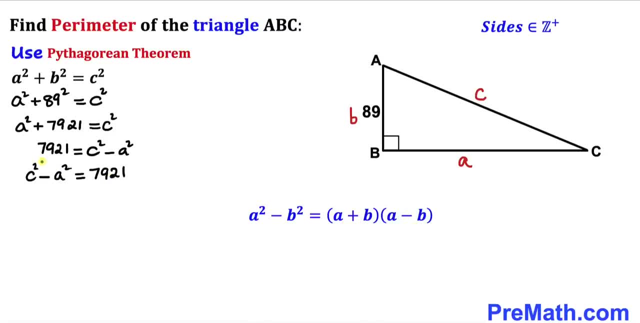 times a minus b, and we are going to apply this identity on the left hand side. so therefore we can write this left hand side as c plus a times c minus a, equal to 7921. and now let's focus on the left hand side. we got two factors, so therefore we are going to: 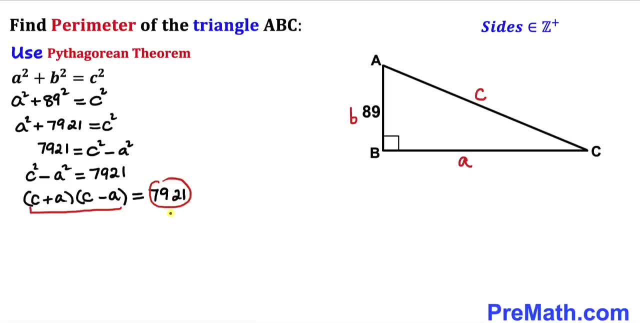 write this right hand side as a product of two factors as well. so first scenario is going to be: we can write 7921 as 7921 times one, and the other option is 7921 could be written as 89 times 89. so let's go ahead and write down this left hand. 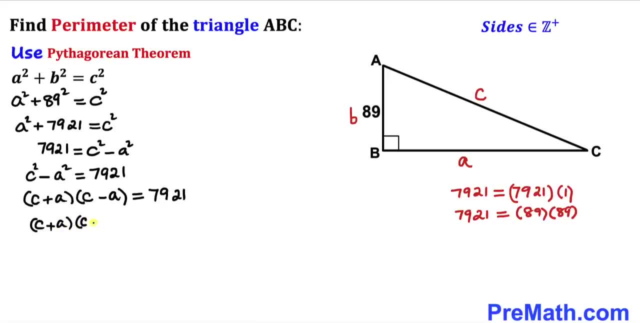 side c plus a times c minus a. let's write down the first scenario, which is this one. so i'm going to write down 7921 times one. and let's write down now the second scenario. so that's going to be c plus a times c minus a equals to: 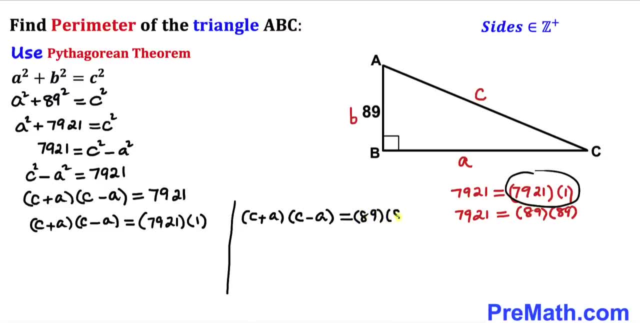 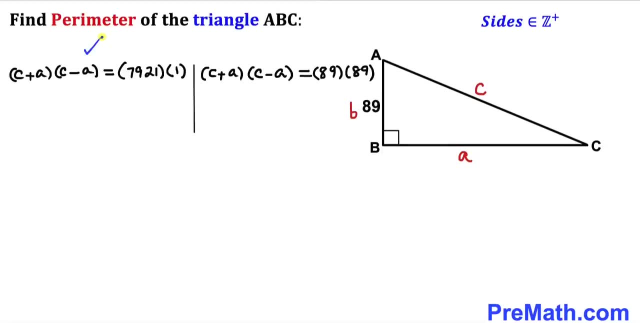 89 times 89. we are talking about this second scenario, and now let's go ahead and focus on this first scenario: c plus a times c minus a, equal to 7921 times one. and we know that c plus a is going to be a bigger number and c minus a is going to be a smaller number. and here this is: 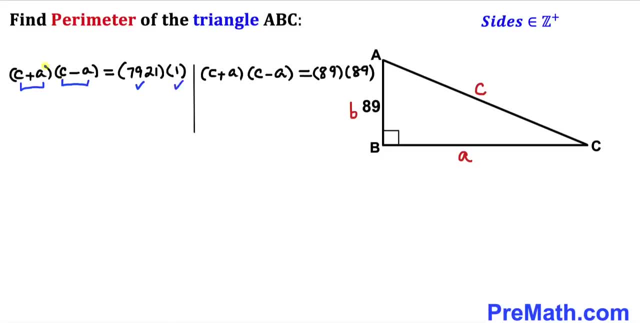 our bigger number and this is our smaller number. so we're going to match c plus a with this one and c minus a with this one. so therefore, we are going to split this one. we can write c plus a equal to 7921, and the other scenario is c minus a equals to 1. and now let's 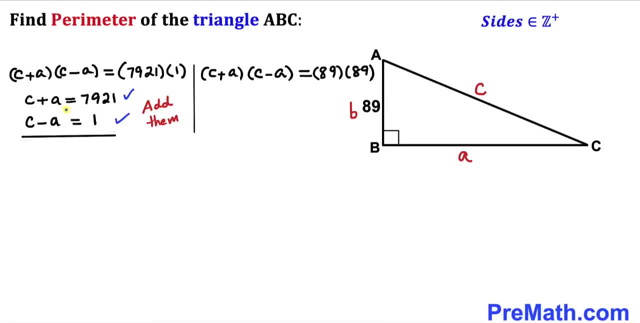 go ahead and add these two equations to eliminate a, we can see this: positive a and negative a is gone. so therefore we're going to get 2c on the left hand side equal to 7922 on the right hand side. let's divide both side by 2, so c is going to be equal to 3961. so we figured out our. 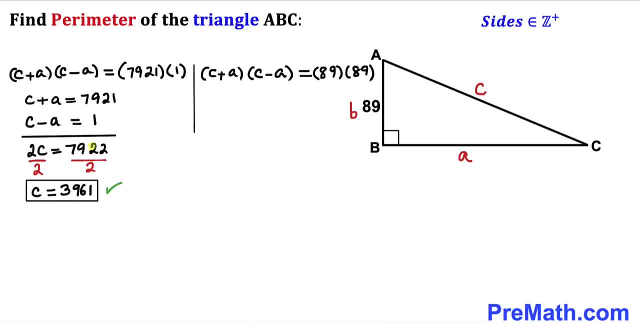 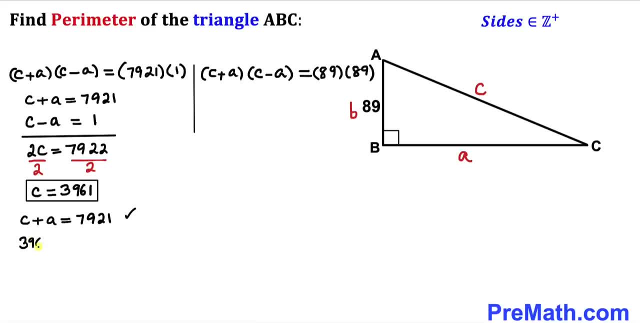 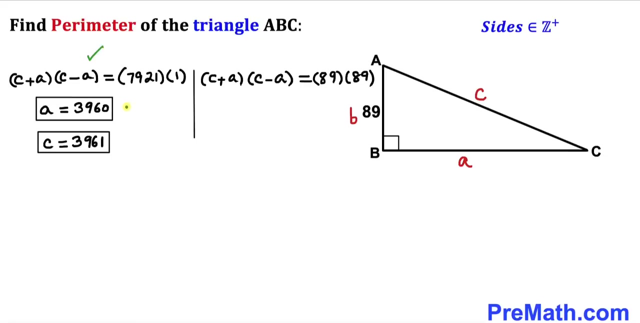 c value as 3961, plus a equal to 7921. and now let's go ahead and subtract 3961 from both sides, this is gone. so, therefore, our a value turns out to be 3960. so thus, for our this first scenario, our a and c value have been calculated. and now let's focus on our this second scenario. we are 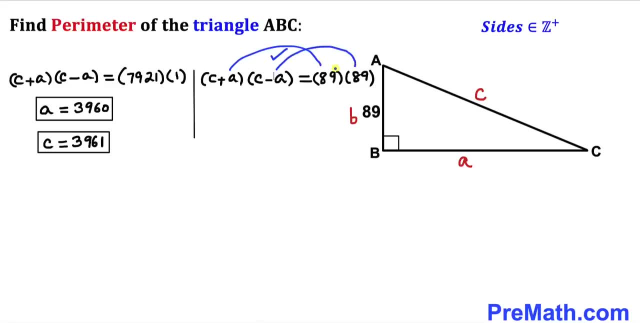 going to equate these two factors. so therefore i'm going to write down: c plus a equals to 89, and the other one is: c minus a is 89 as well. and now let's go ahead and subtract the second equation from the first one. so i'm going to change the sign. this become negative. 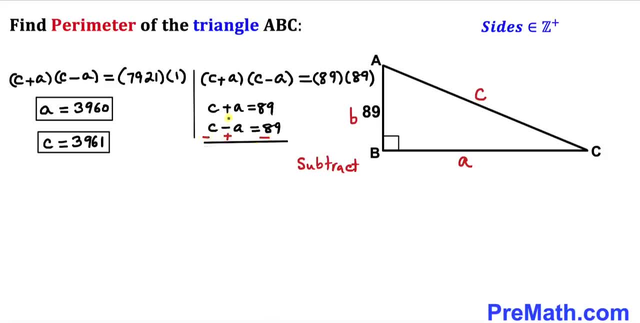 this become positive, this become negative, and we know this. c and negative c, they are gone. so we ended up with the 2a on the left hand side equals to 89 minus 89 is going to give us 0. let's divide both sides by 2, so therefore a value turns out to be: 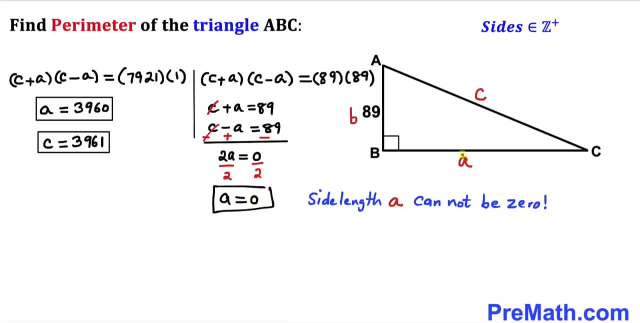 0, and now we can see that our this side length a, cannot be equal to 0. so therefore we are going to reject this, our second scenario, and we are going to accept our first scenario. so that's our a value. i'm going to write down over here: 3960, and our c value is going to be: 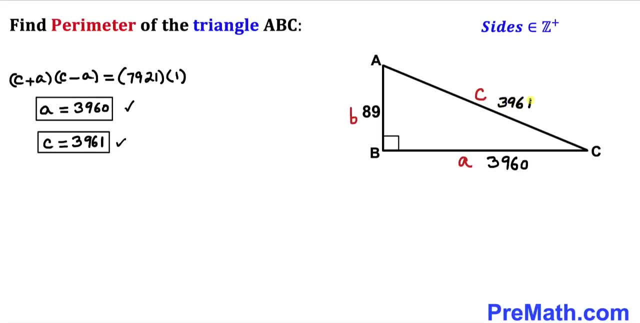 3961. and here's our final step. let's go ahead and calculate the perimeter of this right triangle abc now. and we figured out our all these side lengths. our a value is 3960, b value is 89 and c value is 3961. so let's go ahead and 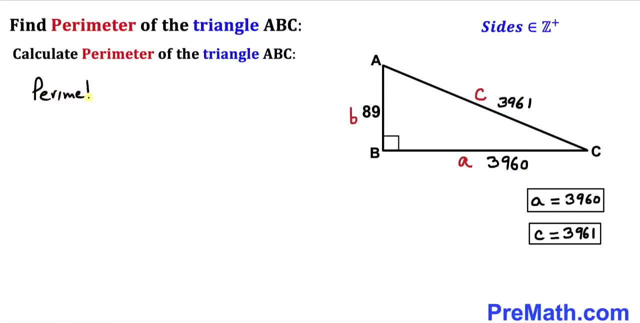 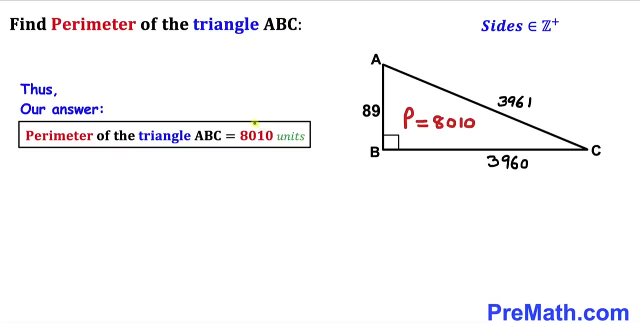 calculate the perimeter of this triangle by just adding all these numbers. our a value is 3960, plus b value is 89, plus c value is 3960 and if we add everything on the right hand side, these numbers, we are going to get 8010. so that's, the perimeter of this triangle turns out to be 8010 units. thanks for watching. 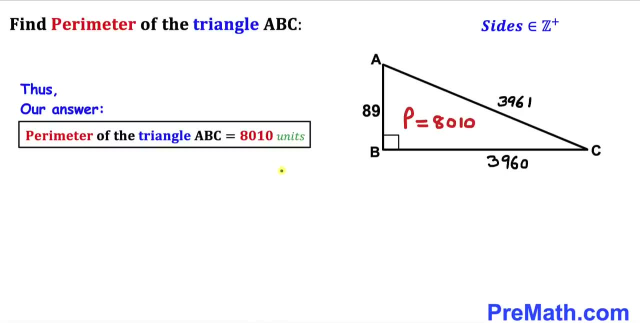 it. please don't forget to subscribe to my channel for more exciting videos. bye.